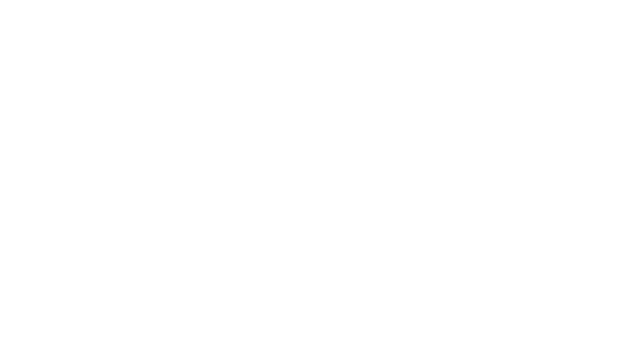 said to be in the s domain or the complex frequency domain. So basically, we select a function and then we transform that function from the time domain to the complex frequency domain. So, given the function f of t, which is defined for all values of t greater than or equal to zero, 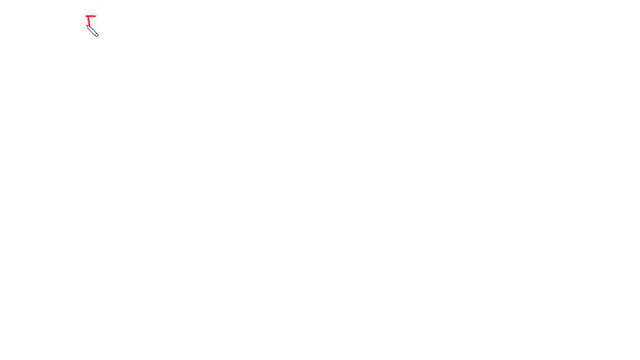 the Laplace transform of that function is given by f of s is equal to. we have the improper integral from zero to infinity, of e, to the power negative s, t times f of t, the t for all values of s for which the improper integral converges. So two conditions for the 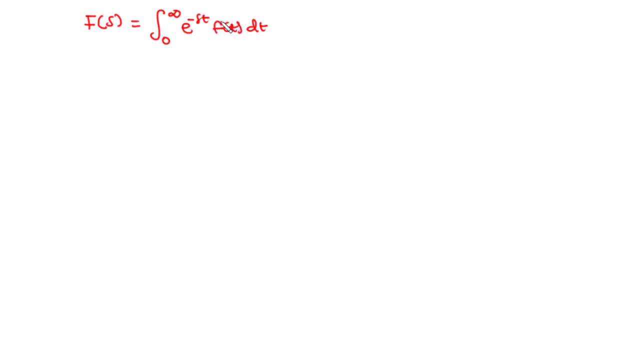 Laplace transform to exist One. we say that the function f of t should be defined for all values of t greater than or equal to zero, or should be defined in the interval close bracket, zero comma plus infinity, Open bracket. And then, secondly, the improper integral must also converge. 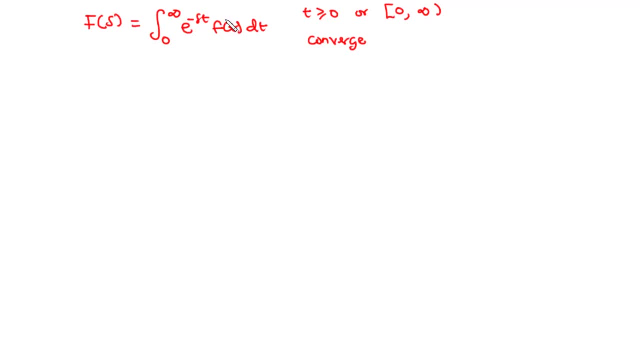 So basically, if you look here, you realize that we plug in a function of t and then we obtain a function of s. So we plug in a function of time and then we obtain a function of s. Now the Laplace transform of the function f of t, which is given as f of s and is equal to the: 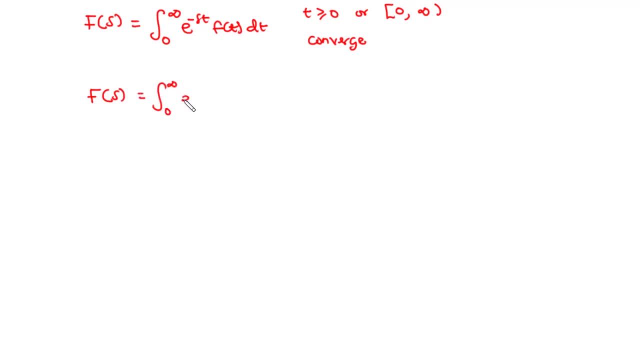 improper integral From zero to infinity of e to the power negative s? t times f of t, the t can as well be represented as we are going to take the limit as m approaches infinity of the integral from zero to m of e to 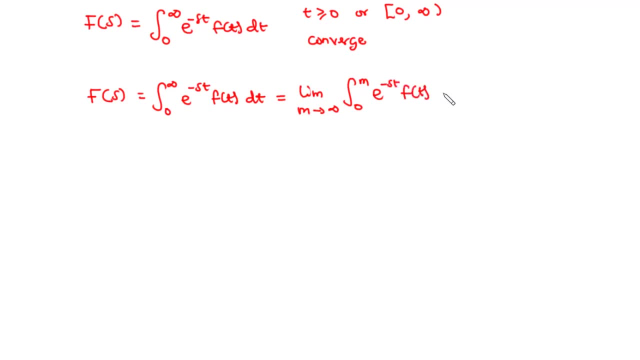 the power negative s t times f of t, the t. Now the reason why we want to take the limit as m approaches infinity is that, in actual sense, you cannot evaluate the limit as m approaches infinity. What we can only do is to take the limit approaching infinity. 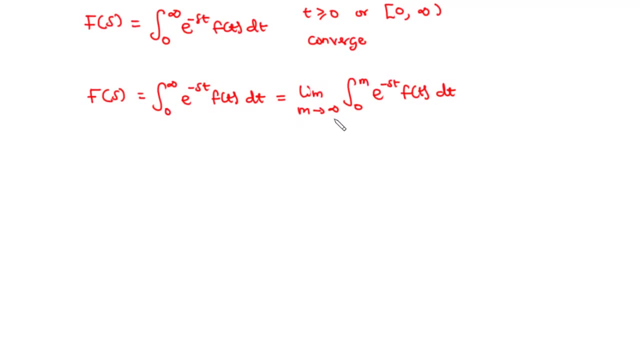 That is why we take the limit as m approaches infinity. Now we need to understand that there are some functions that usually occur in nature. We have examples as exponential functions, sine functions, cosine functions and the like. Now what we are going to do here is to select at least one or two of these functions that usually 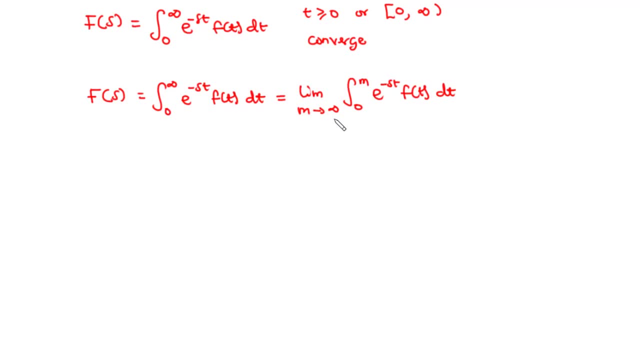 occur in nature and then we try to derive the Laplace transforms. So the first function is the Laplace transform. So the first function is the Laplace transform. So the first function we are going to start off with is the function, that is, the exponential. 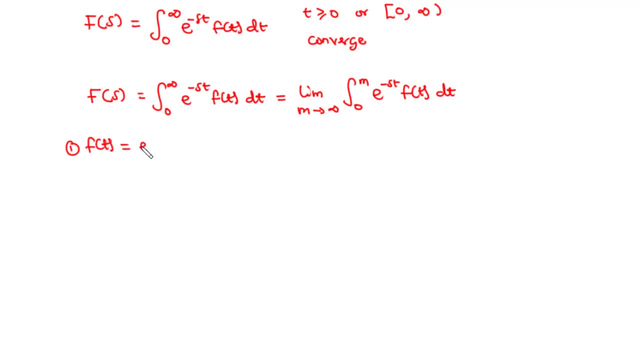 function f of t, and that is equal to e, to the power a, t. So let's start off with this exponential function. So we can as well represent the Laplace transform of a function as we have l, and then we have 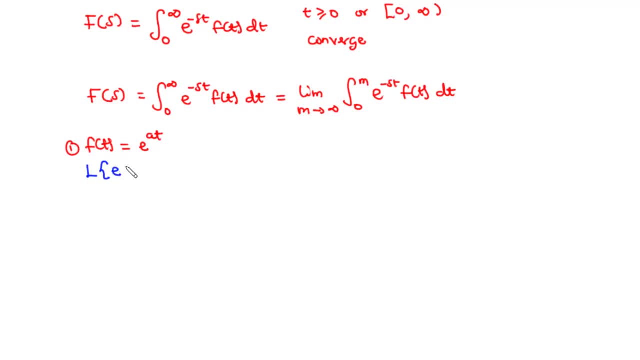 the Laplace bracket of the function. and then we have e to the power, a, t. So this is equal to. we have the improper integral from zero to infinity, of e to the power negative s, t times, f of t, d, t. 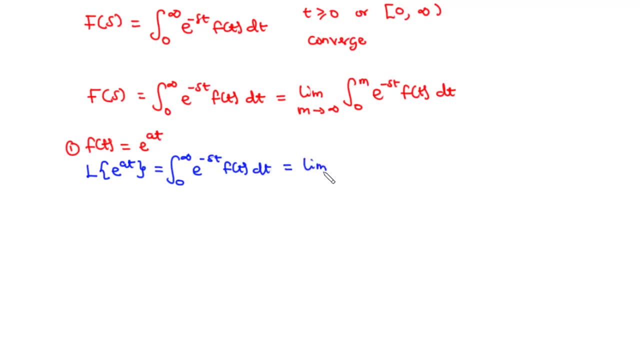 And this is equal to. we have the limit, as m approaches infinity, of the integral from zero to m, and then we have e to the power negative s t times f of t, which is e to the power a, t, d, t. Now let's try to- I mean, solve this. 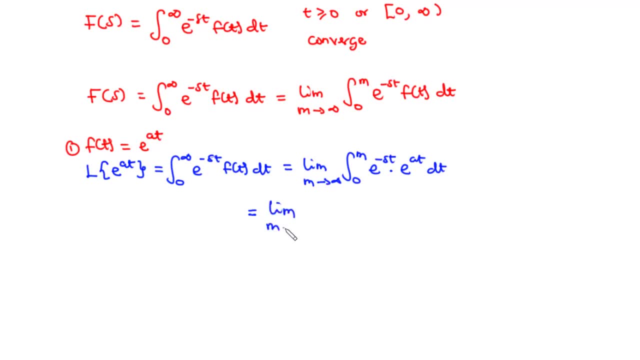 So we have the limit, as m approaches infinity of, we have the integral from zero to m, and then let's try to, I mean, simplify this. So we have the basis to be the same. So we have e to the power. now we have negative or minus on the outside. 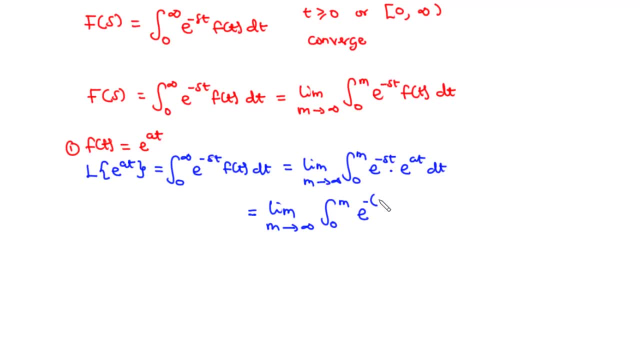 So negative 1 times s is negative s, So we have negative 1 times s. and then negative 1 times negative a gives a, So we have negative 1 times negative a gives a, So that becomes minus a, and then all times t, d, t. 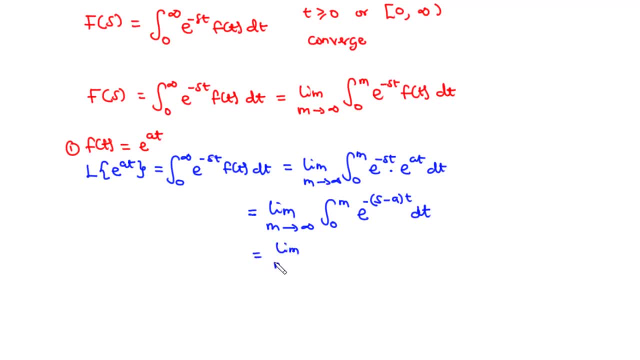 Now the next thing we are going to do: we take the limit as m approaches infinity and then we try to integrate this function. So we are going to have now to integrate this. we can take this as having the integral of e to the power negative 2, t, d, t. 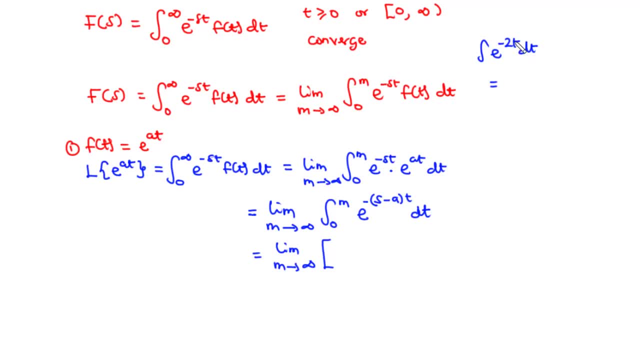 To integrate this. what we are going to do is you are going to first of all rewrite what you have here, that is, e to the power, negative 2 t, and then you differentiate the exponent with respect to t. So derivative of negative 2 t with respect to t is negative 2,. 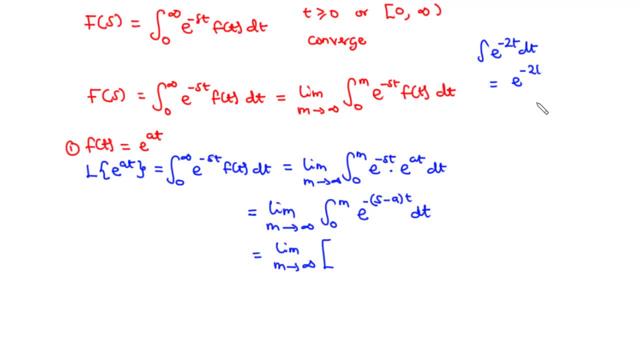 and that negative 2 appears at the denominator. So that is exactly how we are going to treat this. So, first of all, we have e to the power. negative bracket. bracket open s minus a bracket closes t divided by now because we are going to integrate with respect to t. 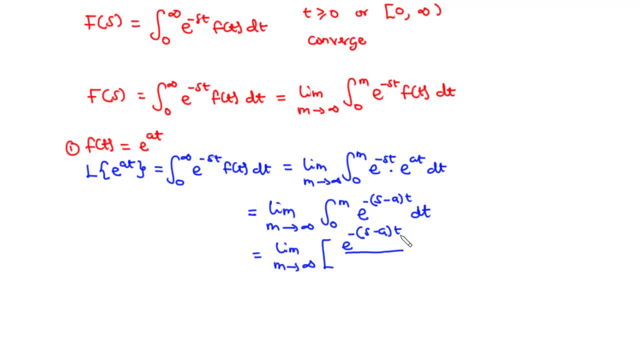 negative into bracket s minus a becomes a constant. So when you integrate the exponent, you have negative s minus a. that is from 0 to m. Now let's continue. So this becomes- we have the limit as m approaches infinity of. 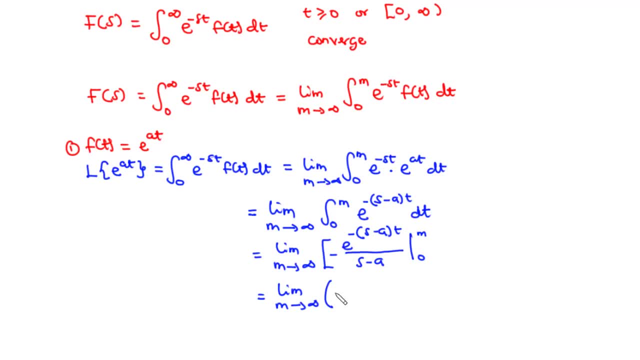 we simplify this or we try to represent it in a more nice way. So negative 1 over s minus a times. now we are going to evaluate the upper limit minus the lower limit, So we have e to the power. negative into bracket s minus a. 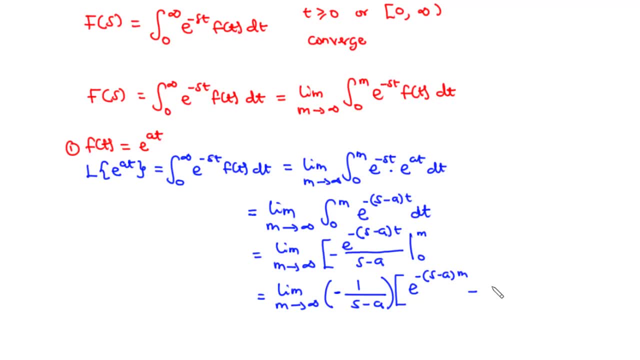 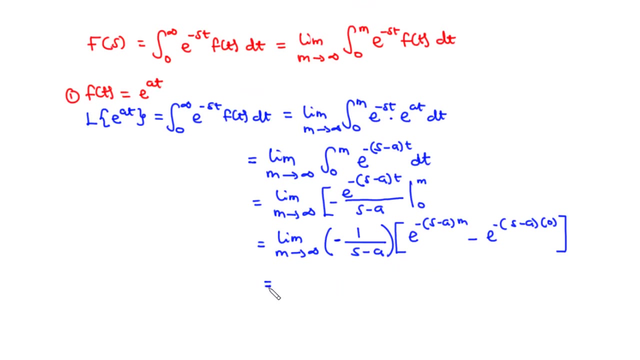 and then, in place of t, we have m minus e to the power negative into bracket s minus a. in place of t we have zero. Now, in the next step we are going to do, we are going to do two assumptions. 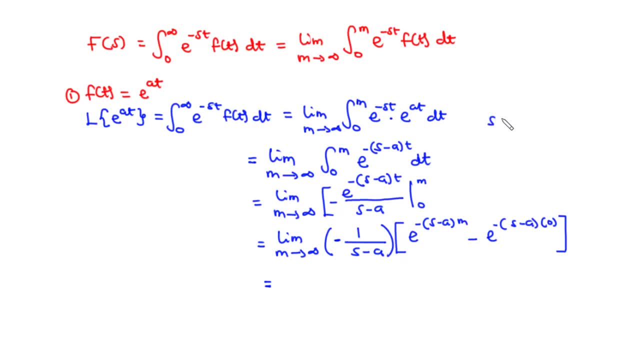 So, first of all, we are going to assume that s is greater than 0 and then m approaches infinity. So these are the two assumptions we are going to make, And then we are going to have negative 1 over s minus e. 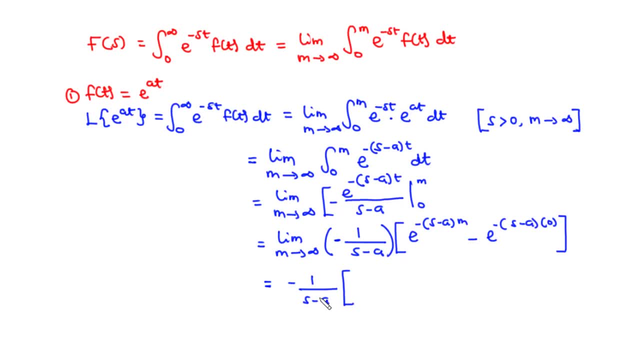 So the limit goes away, and then we have this fraction multiplying Now as m approaches infinity, and then s greater than zero. we have what's in the bracket to be a positive value and then times infinity, which is also positive, and then times negative, which is negative: infinity. 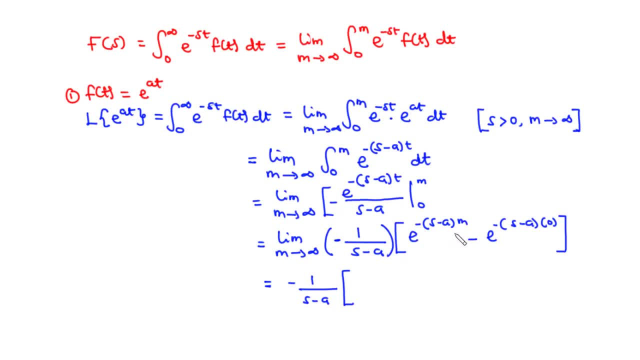 Now e to the power- f value, which is very close to negative infinity, is equal to zero, minus here, because we have zero here. So the exponent becomes zero. and then e to the power: zero is equal to one. Now let's try to multiply the two values. 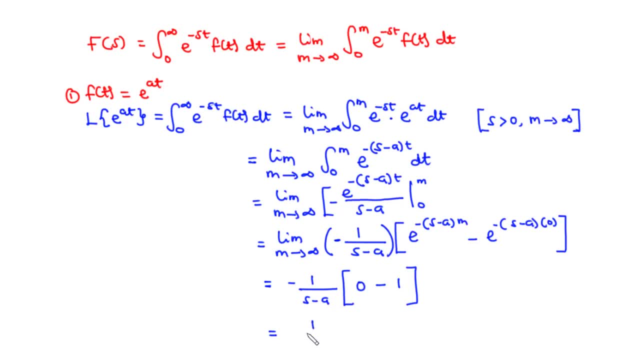 So we have negative. negative it becomes positive. and then we have one over s minus a where s is greater than a. Therefore the Laplace transform of the function e to the power a, t is equal to one over s minus a where s is greater than a. 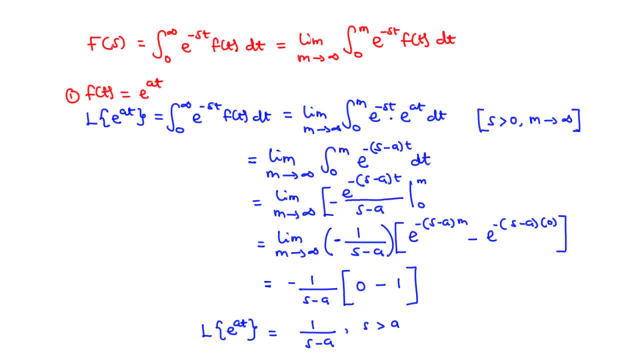 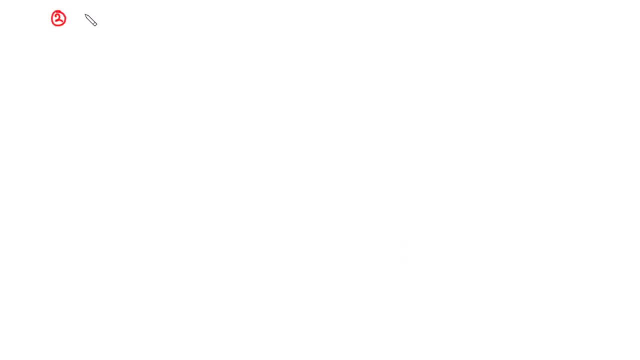 Okay, So this is the Laplace transform of the exponential function e to the power a, t, and this is how to derive that. Now let's look at the second function. Now, the second function we are going to consider, the function f of t, equals to one. 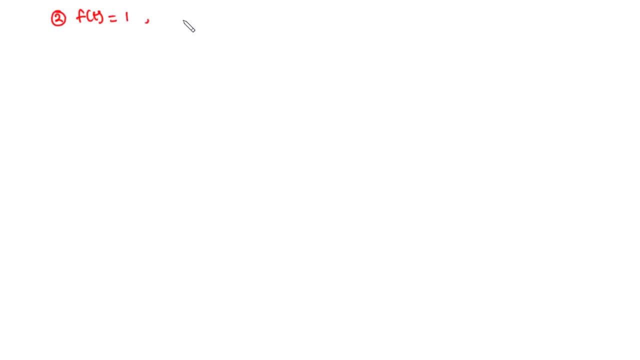 Now, f of t equals one is a special case of e to the power a t, where a is equal to zero. Now if a is equal to zero, we have the exponent to be zero, and then e to the power, zero is equal to one. So the function f of t equals one is a special case of e to the power a t, that is, where a 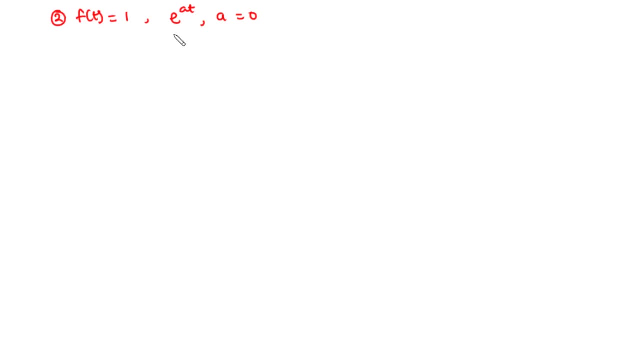 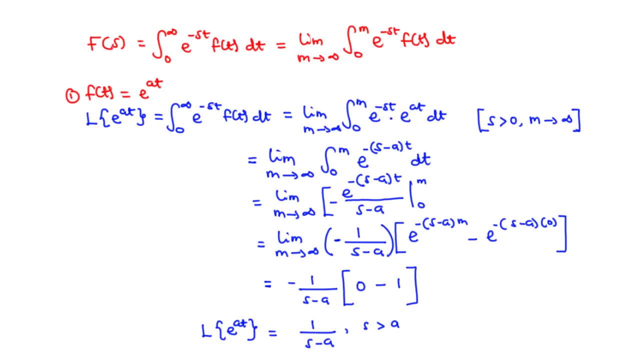 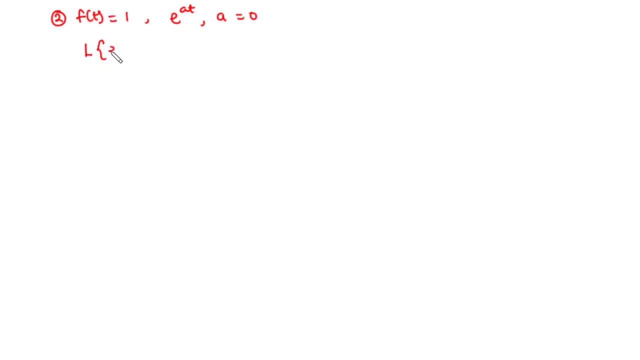 is equal to zero. Now to find the Laplace transform of this function. basically, we are going to use the transform we had in the previous, in the previous function. So we had the Laplace transform, the Laplace transform of the function e to the power a. 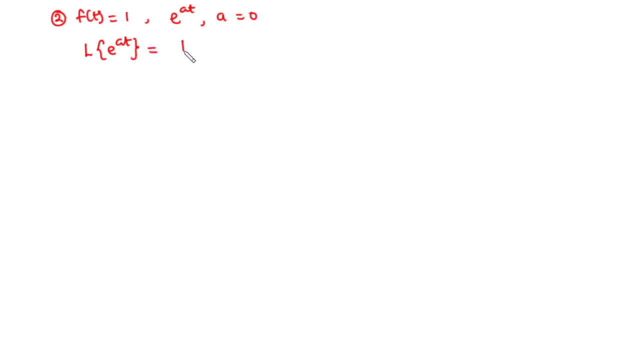 t to the power, a t to be equal to one over s minus a, where s is greater than a. Now, since we have in this case a to be equal to zero, then basically we say that the Laplace transform of one is equal to. we have one over s minus a is equal to zero, so zero and that. 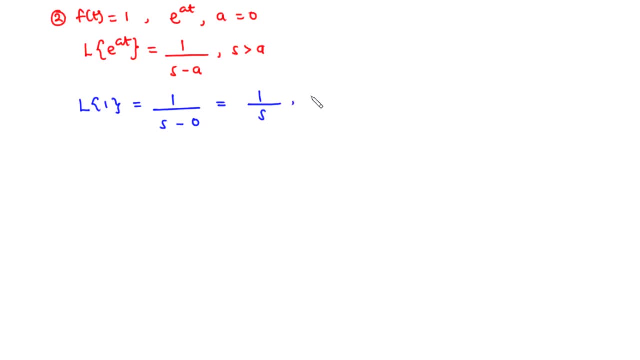 is equal to one over s. Okay, So now we have been able to derive the Laplace transforms of two functions, that is, first f of t equals e to the power a t, and then f of t equals one. Now, aside from these two functions, there are some more functions which also occur frequently. 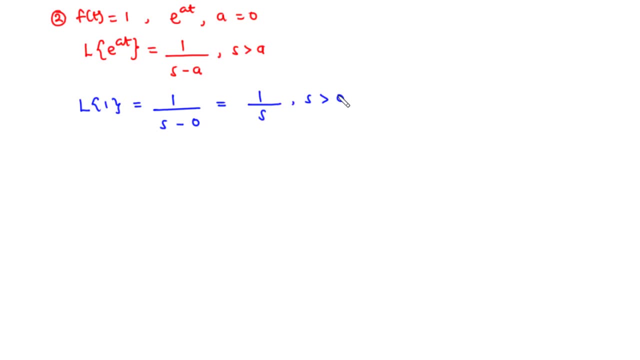 in nature, We are not going to derive such functions. what you are going to do is to construct a table where we have all these functions in there, and then we try to take examples of each form of the function, and that is going to help us to obtain the Laplace transform. 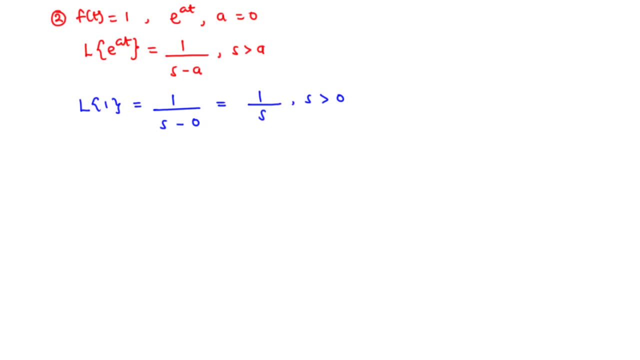 of certain other complex functions. So for now we know two functions with their respective Laplace transforms. So to fill our table, we are going to consider the first function, which is the function f of t equals one, So we have the Laplace transform of one, and then we already know that this is equal to. 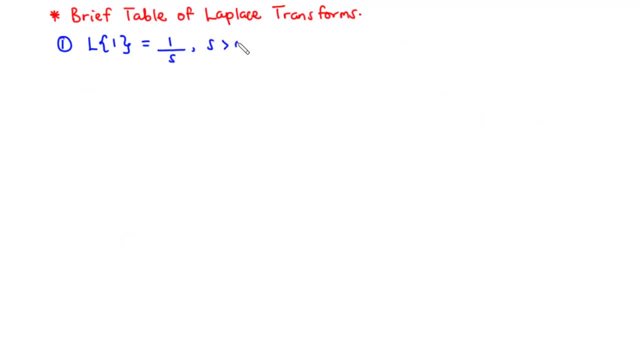 one over s. Okay, Where s is greater than zero. So let's try to find the Laplace transform of. let's say, the function f of x equals two. So how do we find the Laplace transform of this function? Now, before we can solve this problem, we need to know the property of Laplace transform. 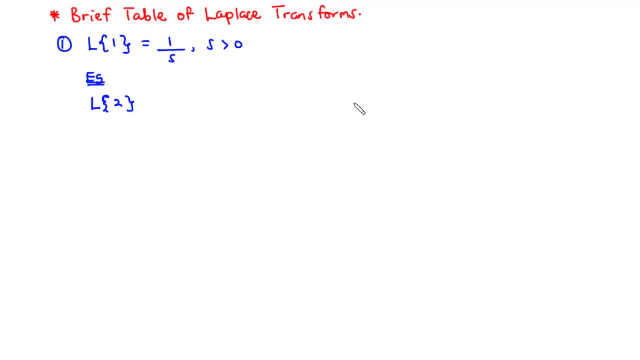 which we call the linearity property, The linearity property. So this is the linearity property. Now, this property states that, assuming we have two functions, f1 and then f2, with two constants, c1 and c2, so that we have the Laplace transform of the function c1, f1 plus c2, f2, 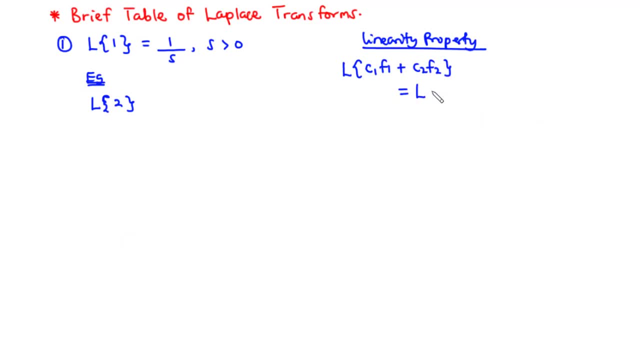 then we can split these two so that we have the Laplace transform of c1- f1, plus the Laplace transform of c2- f2.. Now, because c1 and c2 are constants, we can pull them out so that we have c1, the Laplace. 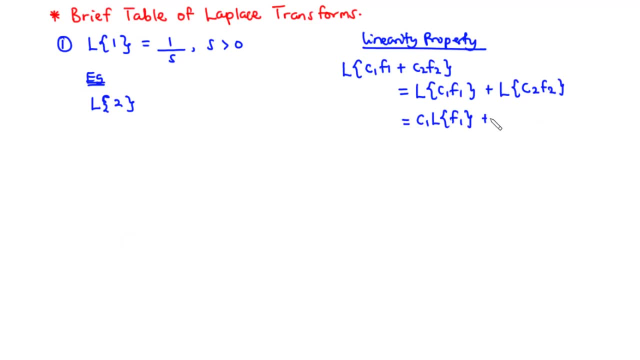 transform of f1 plus c2, the Laplace transform of f2.. So basically, that is what we are going to use here, So we can represent this as the Laplace transform of two times one, And then, because two is a constant, we pull out two. 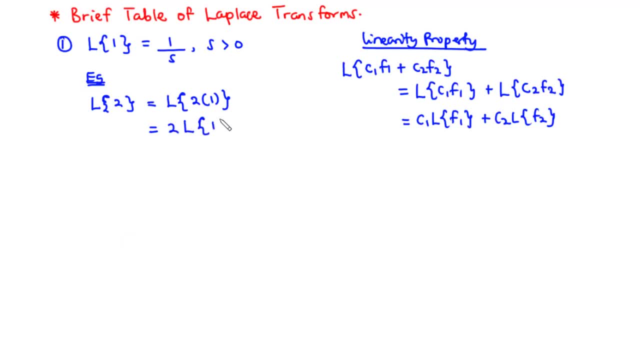 So we have two times the Laplace transform of one, And then we already know the Laplace transform of one as one over s. So we have one over s here. we multiply two across so that we have two over s where s is greater than zero. 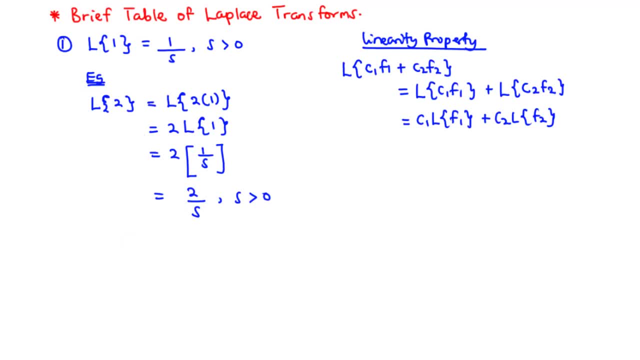 So the Laplace transform of two is equal to two over s. Now let's move on to the second question. So the Laplace transform of two is equal to two over s. Now let's move on to the second question. So the Laplace transform of two is equal to two over s. 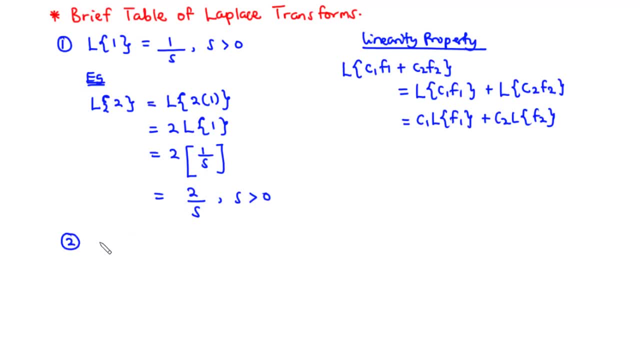 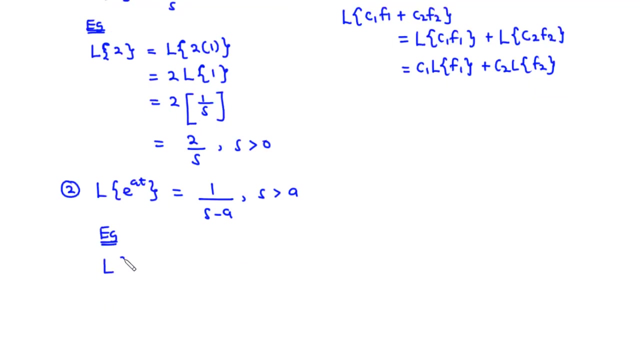 That is the function f of t equals e to the power at. So that is, we have the Laplace transform of the function e to the power at, and that we know is equal to one over s minus a where s is greater than a. So, assuming we want to find the Laplace transform of the function, let's say three: e to the power. 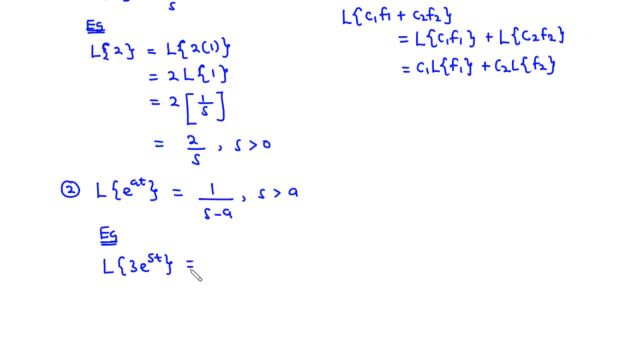 5t. So using the property of linearity of the Laplace transform, we can pull out 3,, which is a constant, And then we have the Laplace transform of the function a to the power 5t. So comparing these two in the Laplace bracket, you realize that we have a to be equal to 5.. 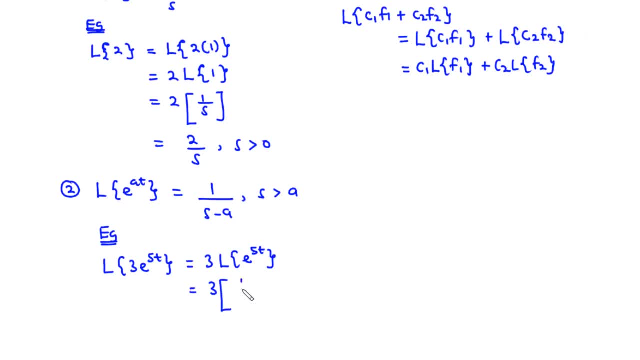 So, using this transform, we have 1 over s minus 5.. And then, finally, we have 3 over s minus 5, where s is greater than 5.. Now let's move on to the third function. We are going to consider the function t to the power n. 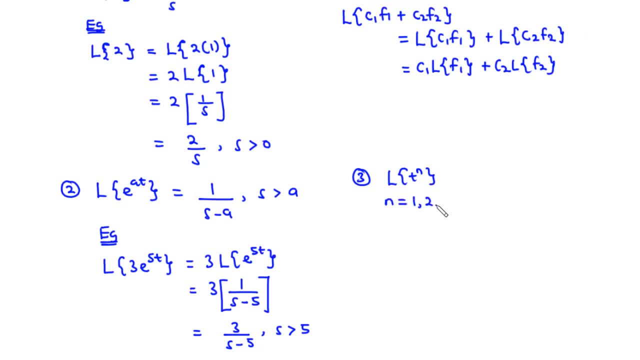 where n is equal to 1,, 2,, 3, and so on and so forth. Now the Laplace transform of this function is said to be equal to n factorial divided by s, to the power n plus 1.. So, for example, if we consider the function t cube, 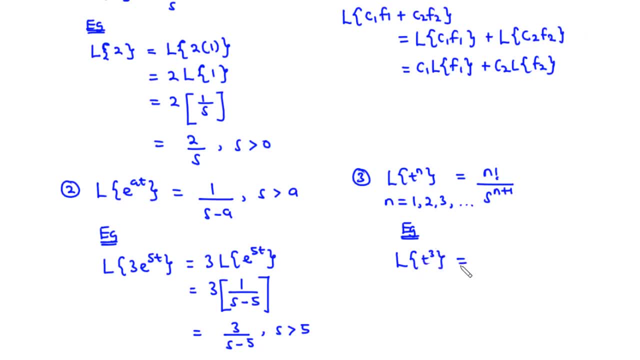 we want to find the Laplace transform of this function. Then we know that n is equal to 3.. So we have 3 factorial divided by s to the power, 3 plus 1.. Now 3 factorial is 3 times 2 times 1, divided by s to the power 4.. 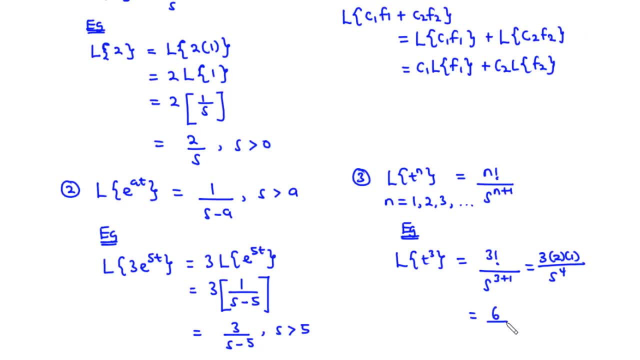 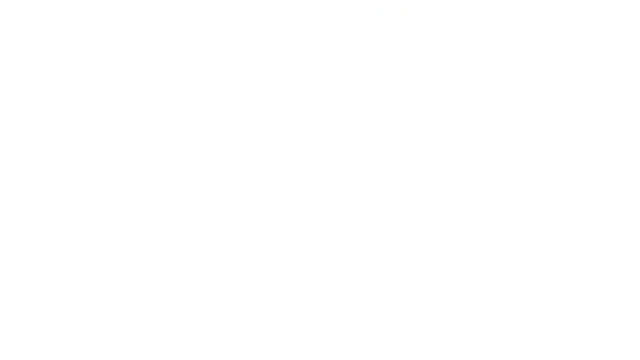 So, finally, we have this to be equal to 6 divided by s to the power 4.. Now let's move on to the fourth function. So for the fourth function, we have the function f of t. We have f of t equals a to the power a t times t to the power n. 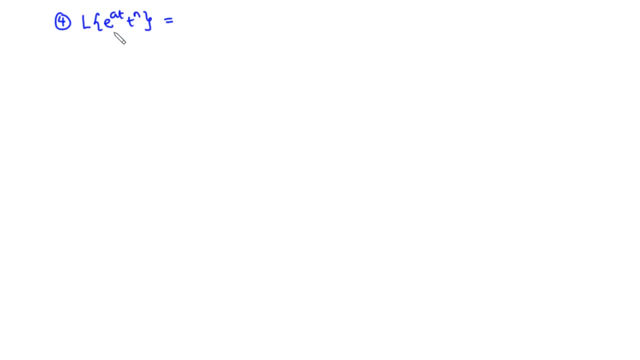 Now this is said to be equal to The Laplace transform of this function, is said to be equal to n factorial over s minus a exponent, n plus 1.. So this is quite similar to the third function. The third function is t to the power n. 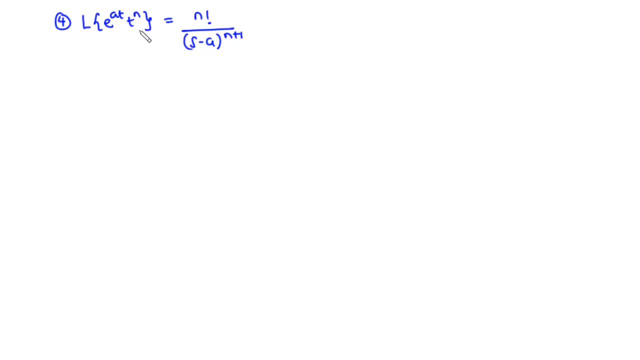 And then this function is e to the power a t times t to the power n. So, taking an example, let's say we want to find the Laplace transform of e to the power 3t times t to the power 2.. 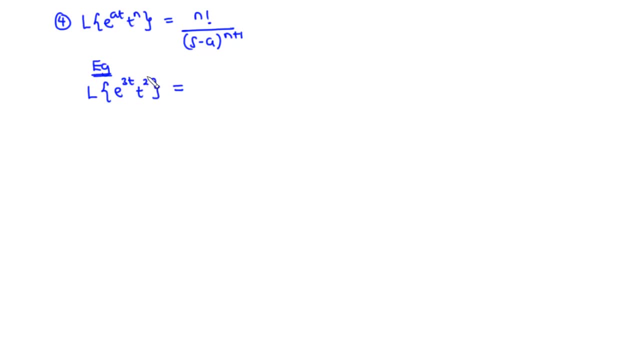 So this will be equal to. We are going to have n factorial, Now t to the power 2 and then t to the power n. Comparing these two functions, you realize that n is equal to 2.. So we have 2 factorial divided by: 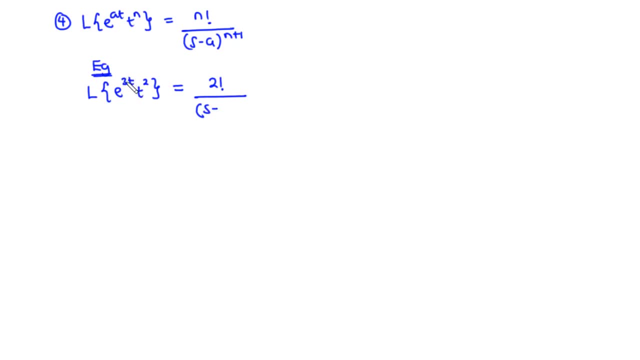 We have s minus a, a is 3.. And then to the power, n, which is 2.. So 2 plus 1.. And then we have this to be equal to 2: factorial is 2 times 1., Which is 2.. 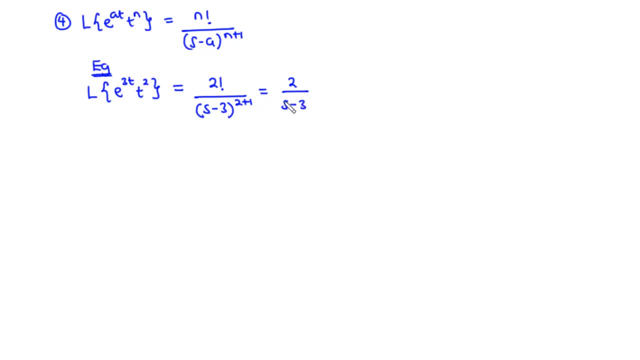 Divided by s minus 3.. exponent 3.. Now let's move on to the fifth function. Now, the fifth function we would like to talk about is The function f of t. equals sine a t. Sine a t. 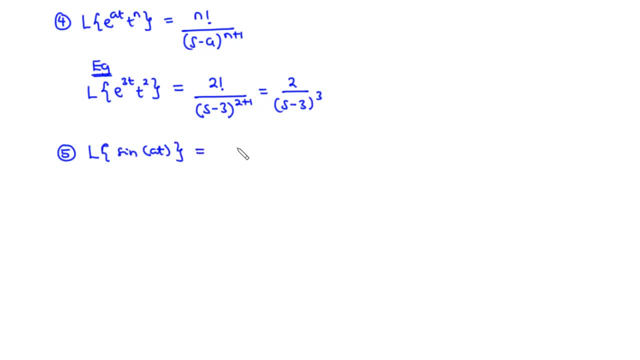 So the Laplace transform of this function is said to be equal to: We have a divided by s squared plus a squared, a divided by s squared plus a squared. Now We are going to take an example. So we want to find the Laplace transform of the function. 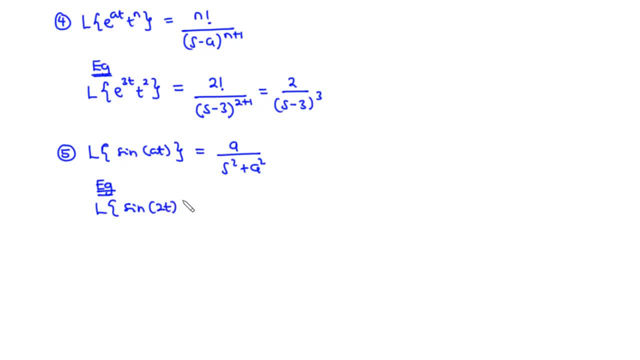 sine 2t, Sine 2t, And this is equal to. Now, the value of a here is 2.. So we have 2 divided by s squared plus a is 2.. So 2 squared, And this is equal to. 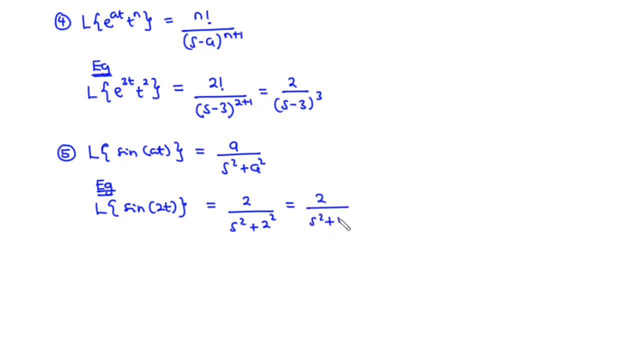 2 divided by s squared plus 4.. Now to the sixth function. We want to find the Laplace transform of the function cos a t That is also given by s divided by s squared plus a squared. 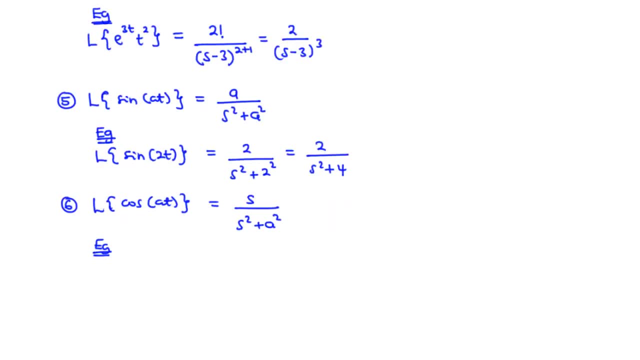 So, taking an example, We want to consider the function cos 2t, So we want to find the Laplace transform of this function. This is also equal to: We have s divided by s squared plus a squared. Now we have a to be 2.. 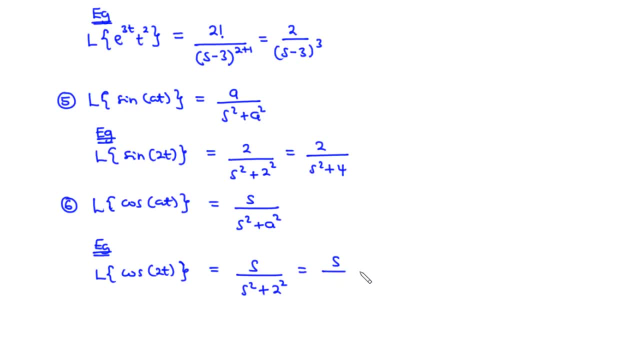 So 2 squared, This is equal to s divided by s squared plus 4.. So note the difference here. If you have the Laplace transform of sin, a, t, That is a over s squared plus. 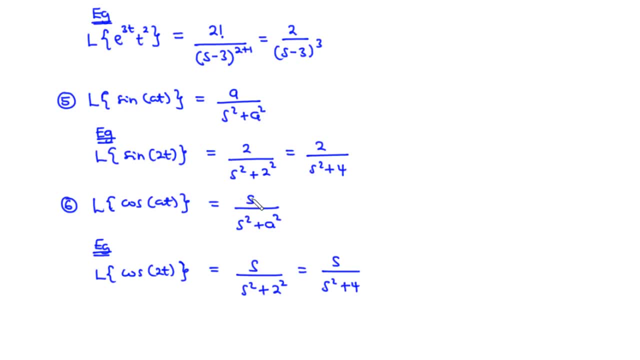 a squared If you have the Laplace transform of cos a t, That is, s over s squared plus a squared. So for sin you have a, For cos you have s. Now let's move on to. 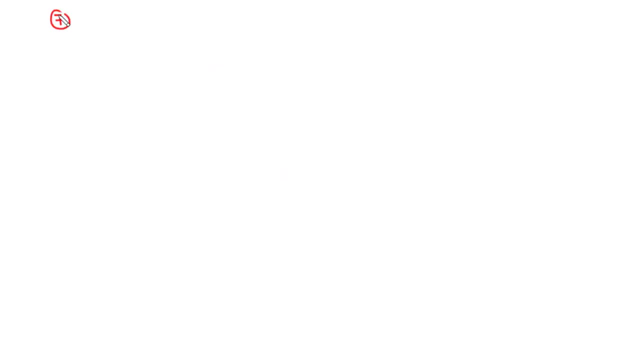 the seventh function. So the seventh function we are going to consider here, We are going to consider the function: f of t equals sin. sin of a, t And that is equal to a divided by. 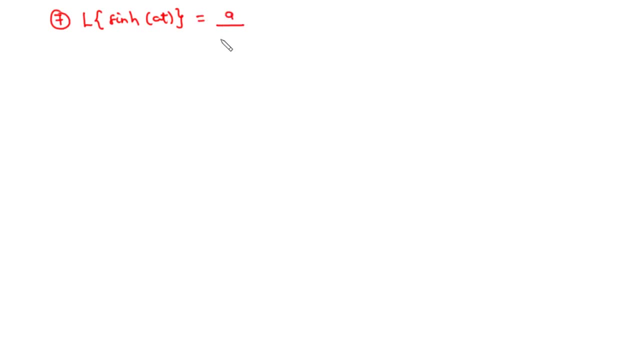 s squared minus a squared Where s is greater than a. So, taking an example, taking an example if you want to find the Laplace transform of the function sin 4t, sin of. 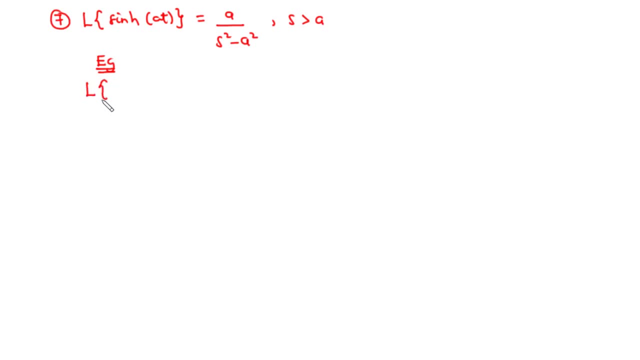 a t. So taking an example, taking an example: if you want to find the Laplace transform of the function 4t, then that is equal to. we have a to be 4.. So 4.. 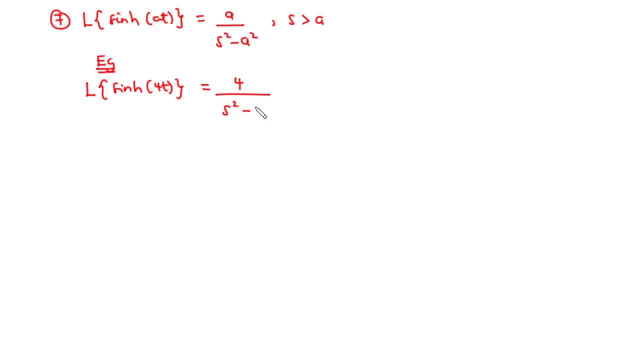 divided by s squared minus a squared, So 4 squared, And that will be equal to: we have 4 divided by s squared minus 16.. Again we move on to the eighth function We have 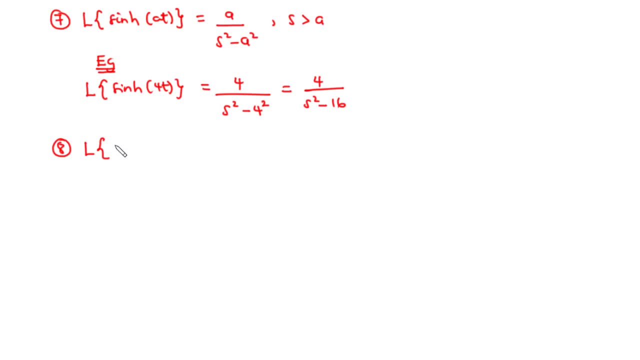 the Laplace transform of the function cos a t of sin 4.. That is also given by s over s squared minus a squared. So we take an example that is: 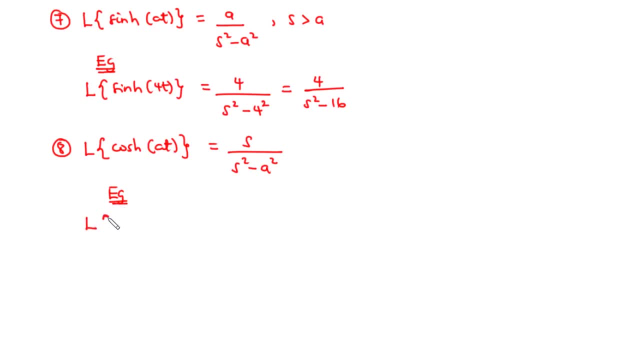 we have the Laplace transform of the function cos 4t. that will be equal to s divided by s squared minus a is 4.. So 4 squared that will also be equal to. 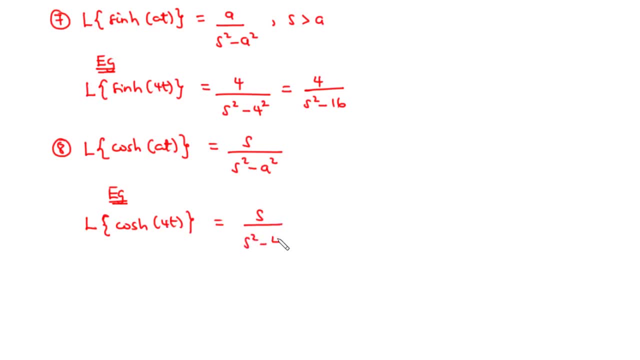 s divided by s squared minus a is 4.. That will also be equal to s over s squared minus 16. Also notice the difference here. Now to the ninth function we are going to consider. 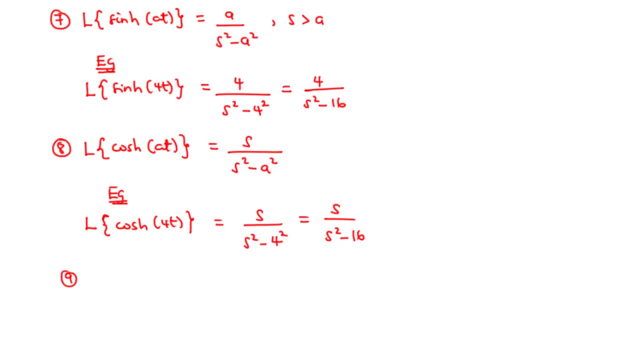 the Laplace transform of the function t sin a t, t sin a t, and that is equal to 2 a s divided by 2 a s divided by 2 a s. 2 a s. 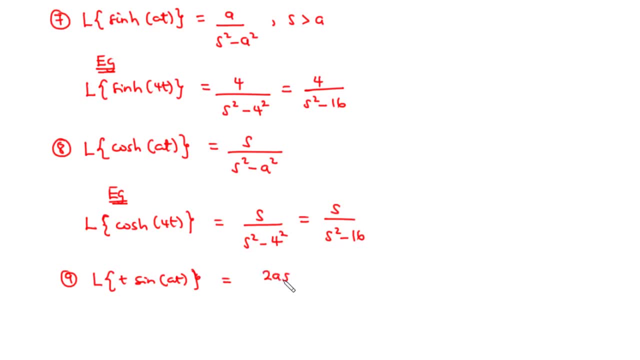 divided by 2 a s, 2 a s divided by a s. 2 a s divided by a s square, a s square plus a square all squared. So taking an example. taking an example. 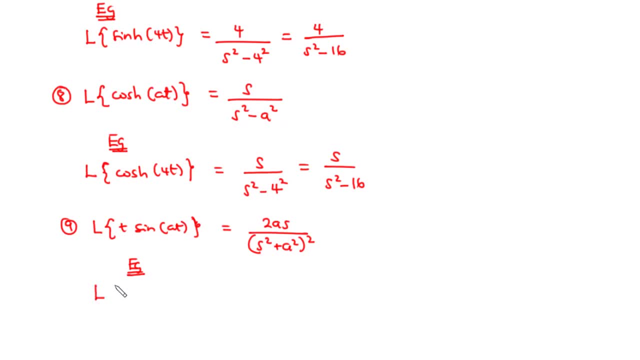 We are going to consider the Laplace transform of the function t, t sin 2t, t sin 2t, t sin 2t. Now this is equal to: we have 2 times a. a is 2, times s divided by the denominator, we have s squared plus a, which is 2, so 2 squared, all squared. 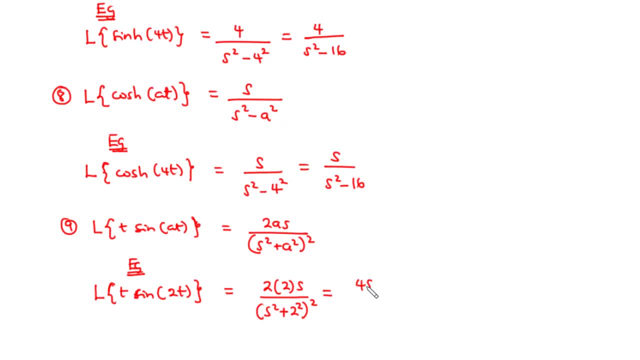 So here this is equal to: we have 4s over s squared plus 4 all squared. So this is the Laplace transform of t sine 2t, t sine 2t. Now let's move on to the 10th function we are going to consider here, that is, we have the Laplace, the Laplace transform of the function. 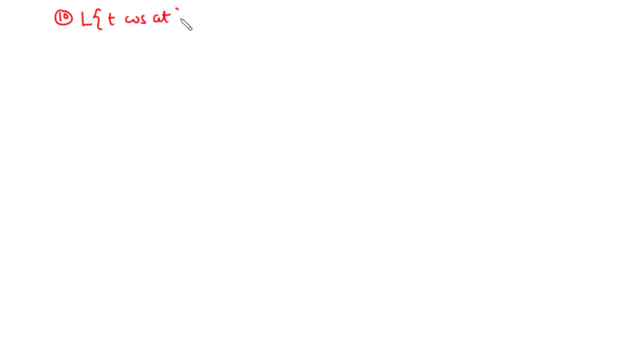 t cos a, t, t cos a t. Now this is given as s squared minus a squared, divided by s squared plus a squared, all squared. We also consider an example, that is, the Laplace transform of t cos 2t. 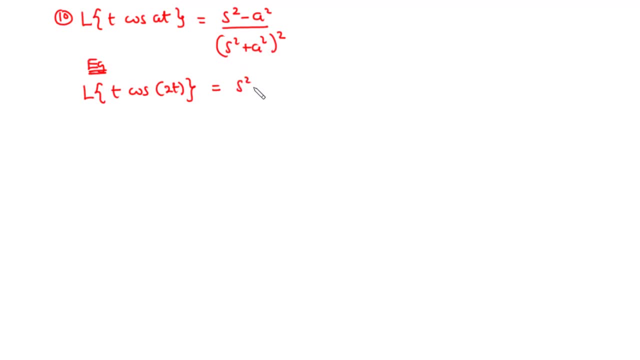 Now let's move on to the 10th function we are going to consider here. that is, we have 4s over s squared plus 4 all squared. This is also equal to: we have s squared minus now a. here is 2, so 2 squared divided by s squared plus a is 2, 2 squared all squared. 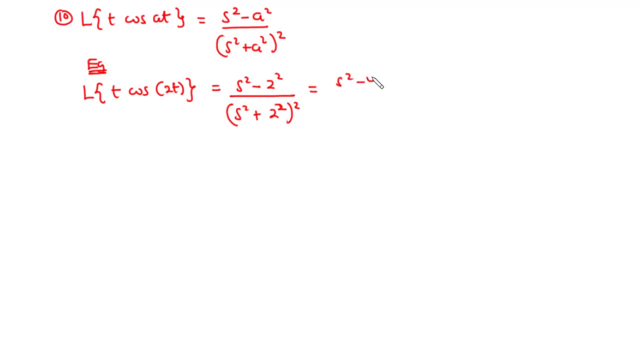 This is equal to s squared minus 4, and then divided by s squared plus 4,, all squared To the 11th function. we consider the Laplace transform of the function sine a t plus b, sine a t plus b. 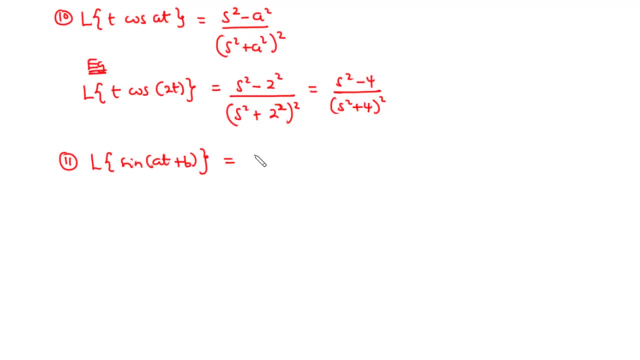 This is nothing but s sine b plus a, cos b, all divided by s squared. So we take the example. we take the example, the Laplace transform of sine 3t plus 5.. We say this is equal to, we have s, and then sine b, b here is 5, so sine 5 plus a. 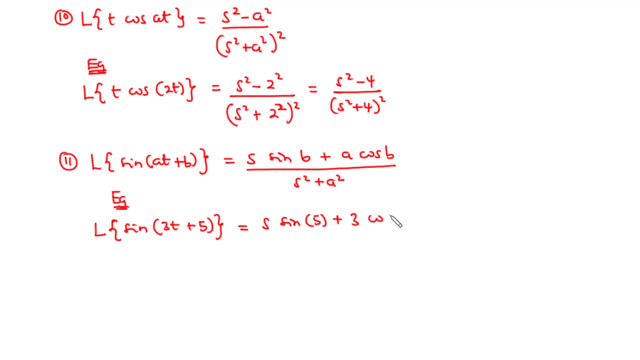 Which is 3, cos b, which is 5, all divided by s squared plus a squared, so 3 squared. Now, 3 squared is equal to 9, so we simply write 9 here. To the 12th function, we have the Laplace transform of this time cos a, t plus b. 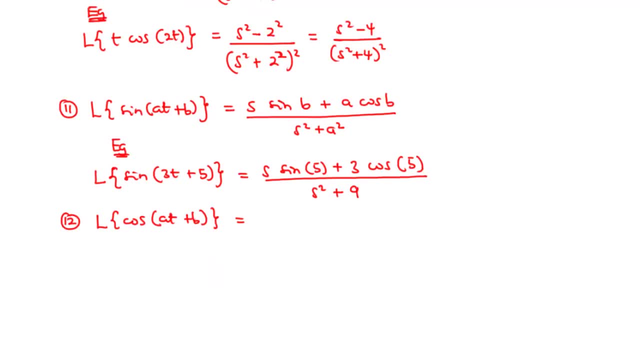 We say this is equal to so with the cos. we are basically going to interchange the positions of sine and the cos and then we negate this operation. so this becomes negative. Instead of addition, it becomes negative. So here we are going to have s cos, b minus a, sine b, all divided by the denominator, remains the same. 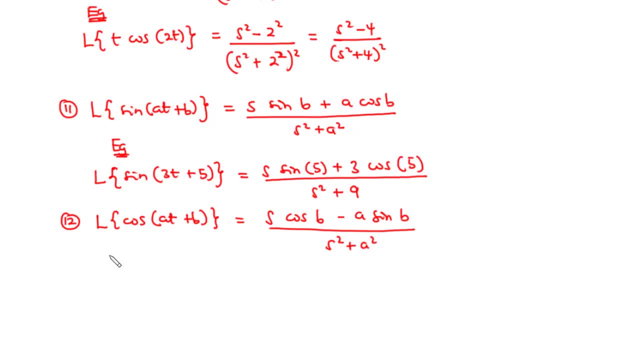 So s squared plus a squared. So, for example, if we consider the Laplace transform of cos 3t plus 5, then here we have s cos b, and then b is 5, minus a, we have a to be 3.. 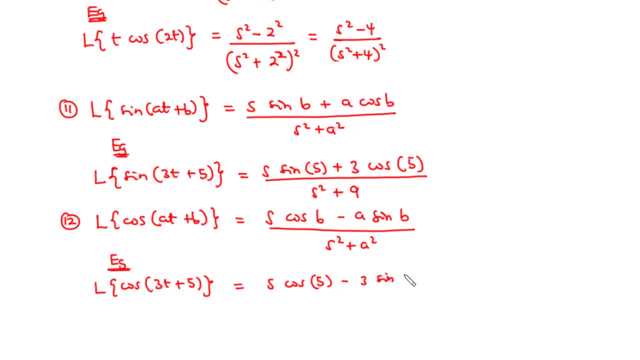 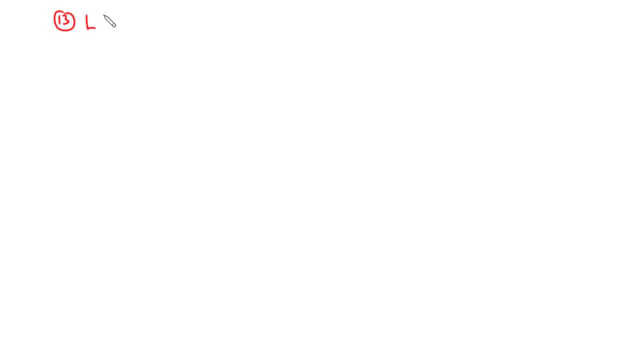 So minus 3.. Sin 5, all divided by s squared plus a, 3 squared. Now, 3 squared is 9, so s squared plus 9.. Now we move on to the last two functions. So we have the 13th function, that is, f of t equals a to the power, a t times sine b, t. 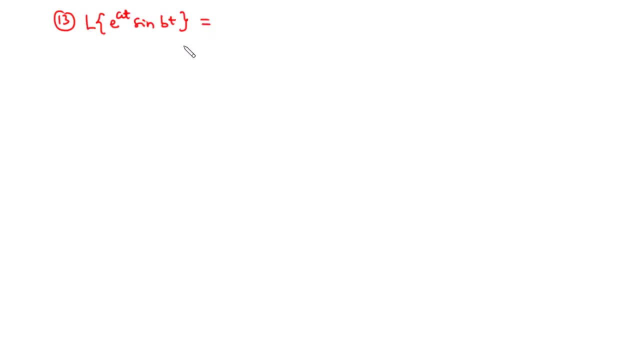 So we want to find the Laplace transform or we want to write down the Laplace transform of this function. Now this is given by b divided by s minus a, all squared plus b squared where s is greater than a. 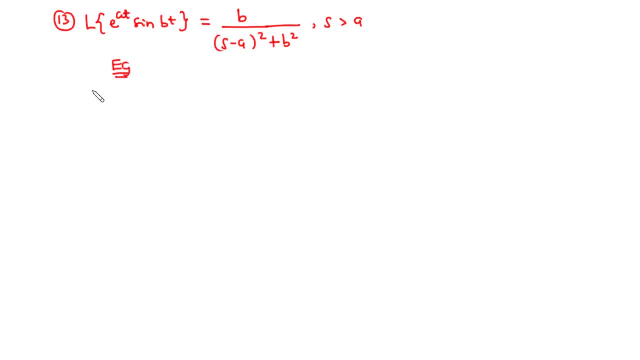 So, for example, we want to find the Laplace transform of the function e to the power 4t sine 5t. So we have b to be 5, so we have 5 on top. and then we have s minus a. a is 4,, so s minus 4,. 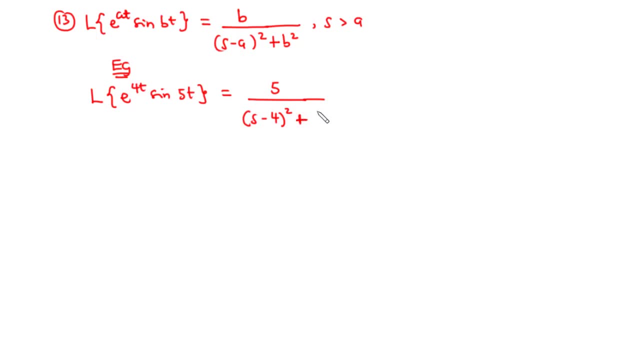 all squared plus b, we know, is 5, so plus 5 squared Now, this is equal to: we are going to have 5 divided by now. let's expand this, So s times 5.. So we have s. we have s squared s times negative 4 is negative 4s. negative 4 times s is also negative 4s. 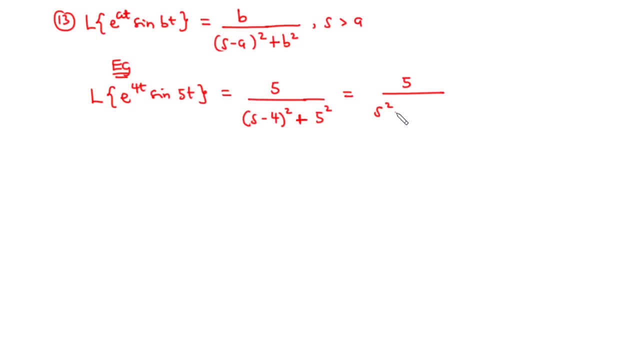 so negative 4 minus 4 is negative 8,. so minus 8s, and then negative 4 times negative. 4 becomes plus 16, and then plus 25.. So finally, we have this to be equal to 5 divided by s squared minus. 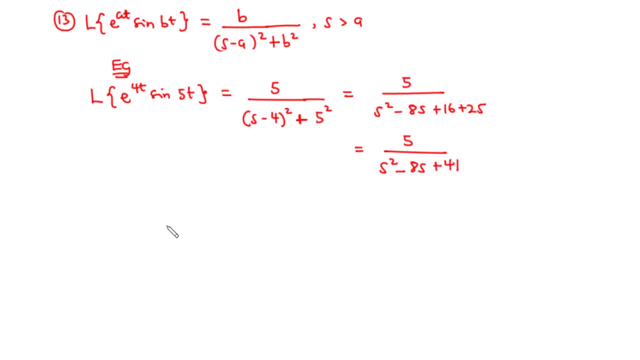 8s and then plus 41.. Now to the 14th function. we are going to take the Laplace transform of e to the power 80,, this time cos bt, and the transform is given by s minus a divided by s minus a. 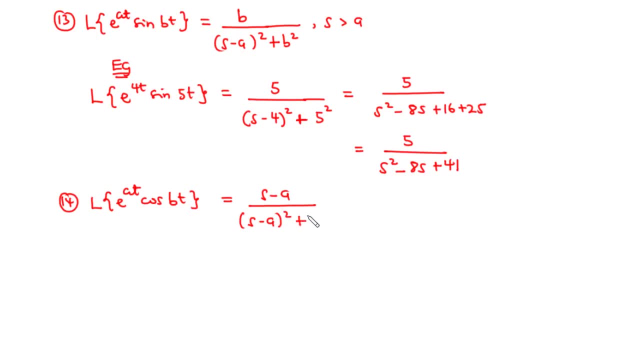 all squared plus b. So this is equal to b squared where s is greater than a. Also, considering the example, the Laplace transform of e to the power 40, cos 5t. so we are going to have: s minus a is 4, so s minus 4, divided by s minus 4, all squared. 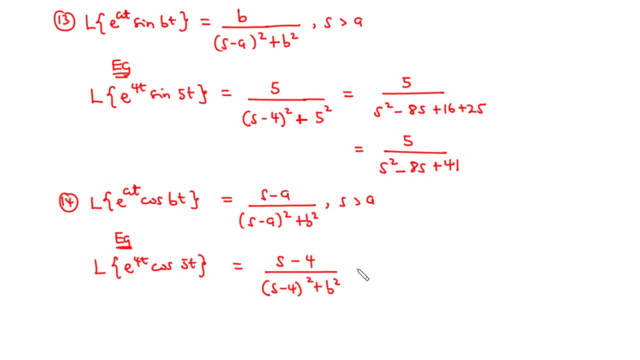 plus b squared. So this is equal to b squared where s is greater than a. So this is equal to: we are going to have s minus 4, divided by so the expansion for s minus 4, all squared gave s squared minus 8s plus 16.. 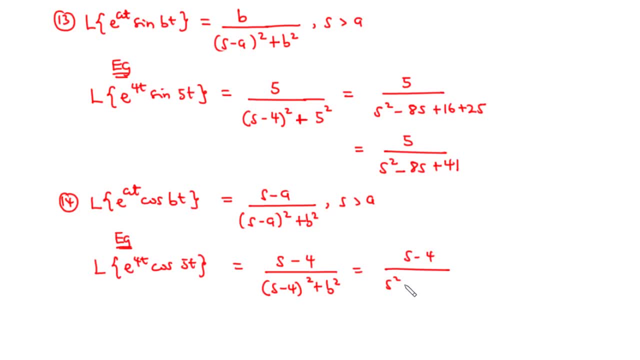 So here we have s squared minus 8s plus 16, and then here we have b, b to be 5.. So 5 squared is 25.. And this is equal to- we are going to have s minus 4, divided by so the expansion for 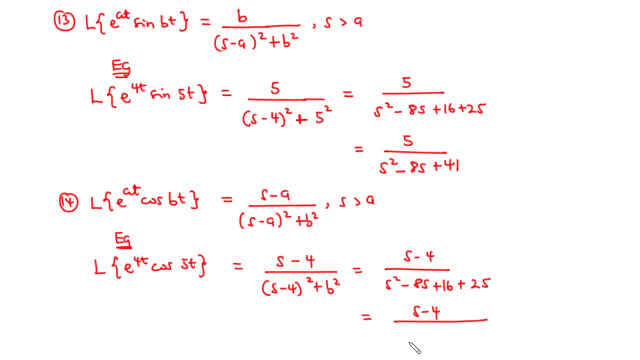 s is equal to s minus 4, divided by s squared minus 8s plus 41.. So that's it for today's video. Now, in the next lesson, we are going to consider the elementary properties of Laplace transform.